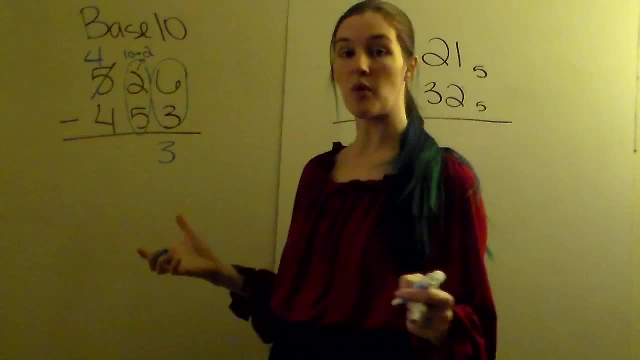 And since our base is 10, we're going to add the base to the base. And since our base is 10, it became a 12.. And it's just easier to write a 1 than to write out. 10 plus 2 equals 12.. 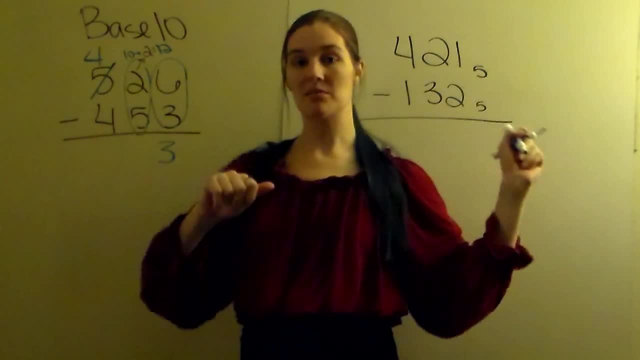 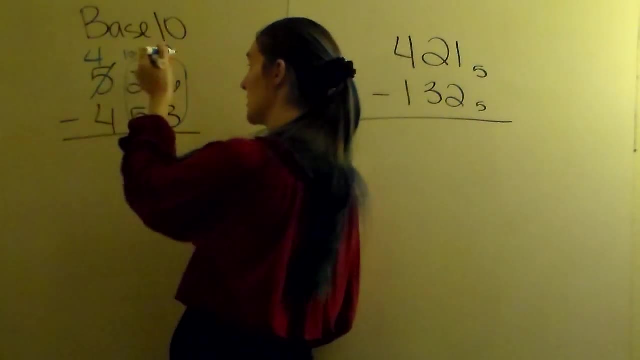 But once we get to base 5, you're not going to be able to just add that 1. You've got to add the base. So when you borrow, always add the base. So 10 plus 2 is 12.. 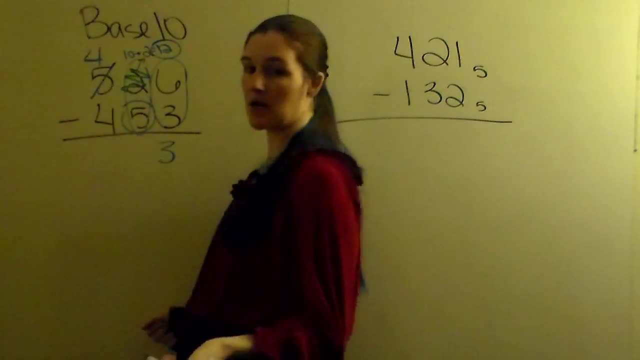 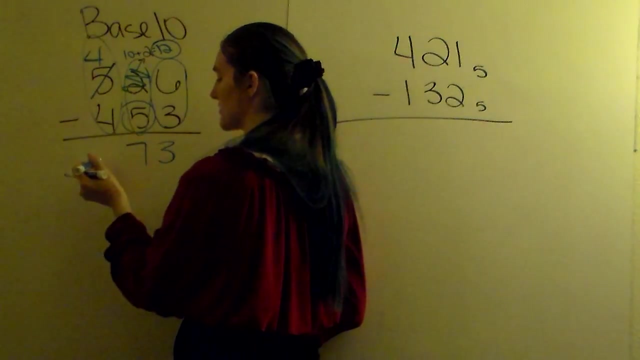 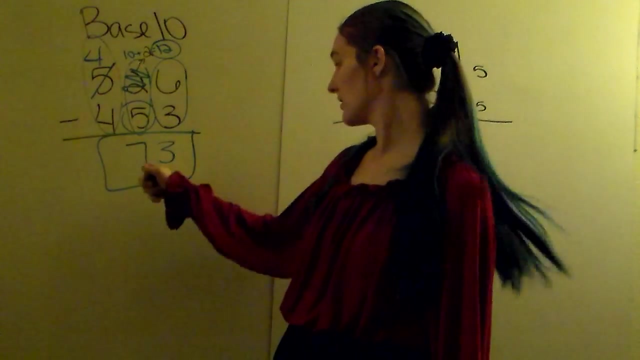 We're going to do 12 minus 5.. The 2 has become a 12.. 12 minus 5 is 7.. Next column is: 4 minus 4 is 8.. 4 minus 4 is 0.. So 526 minus 453 gives you 73.. 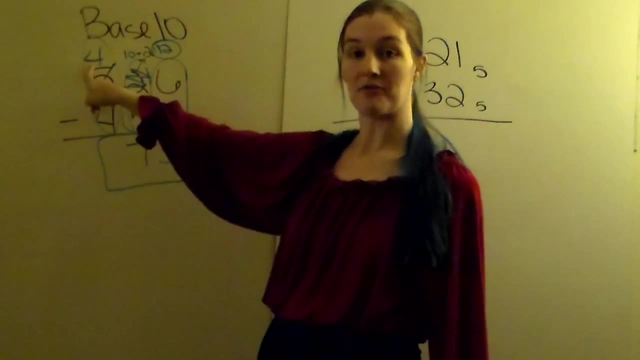 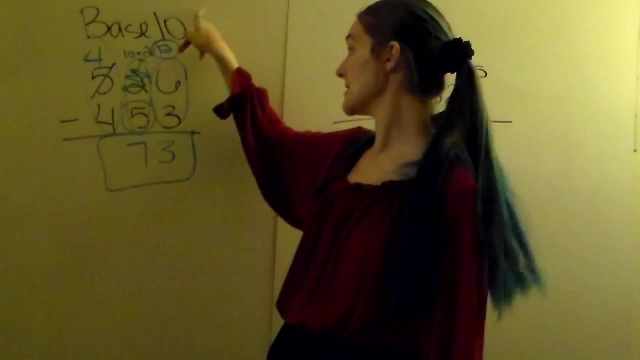 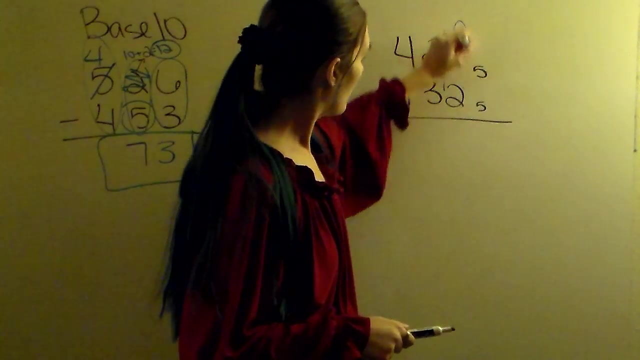 We had to borrow. When you borrow, the number you're taking away from decreases by 1.. The number you're adding to you add the base Base 10, we added 10.. So in base 5, start off the same way. 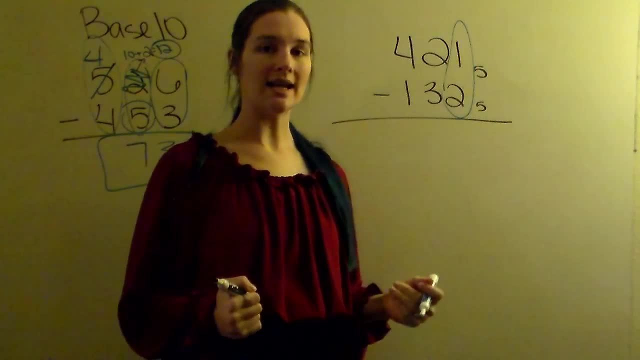 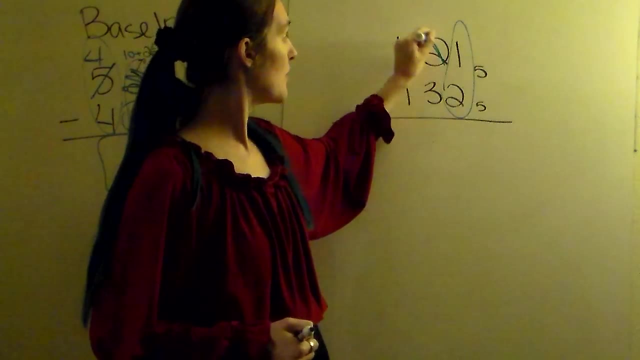 1 minus 2.. That would give us a negative number. We can't have negative numbers, So we're going to go over 1 to the left, giving us the 2.. And we're going to borrow from the 2.. 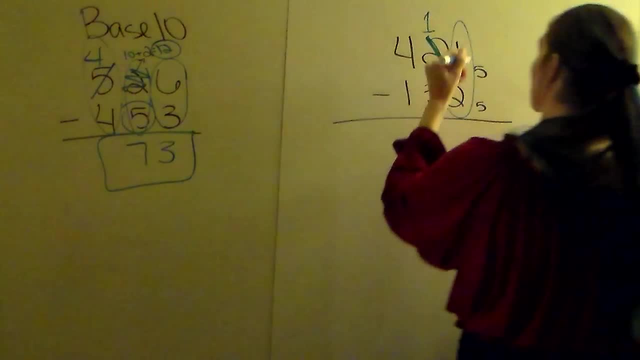 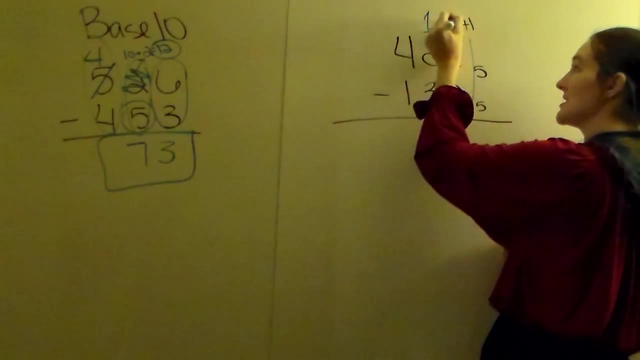 So it's going to become a 1.. And we're going to take this 1 and we're going to add the base to it. So our base, 5 plus 1, is our 6.. We now have 6 instead of 1.. 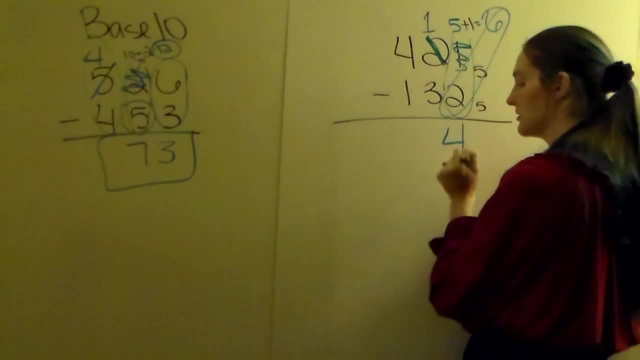 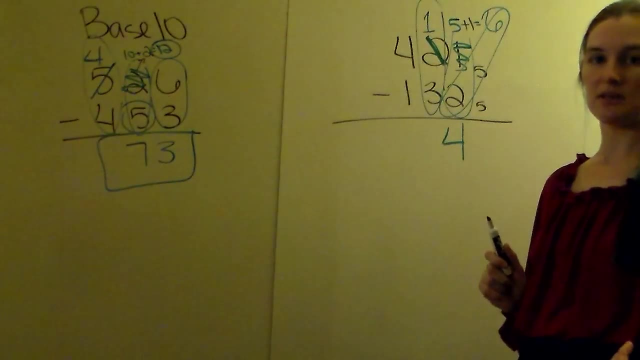 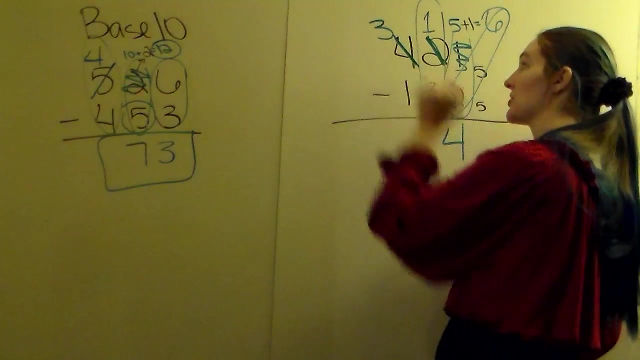 6 minus 2.. We can do giving me 4.. Next column, I'm doing 1 minus 3, would still give me a negative number, So I have to borrow again From the 4, I'm going to take 1 away, making it a 3.. 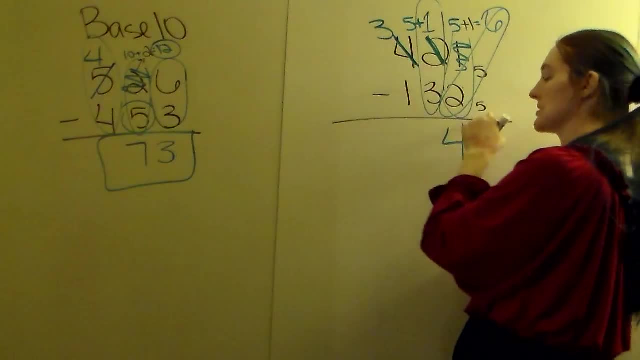 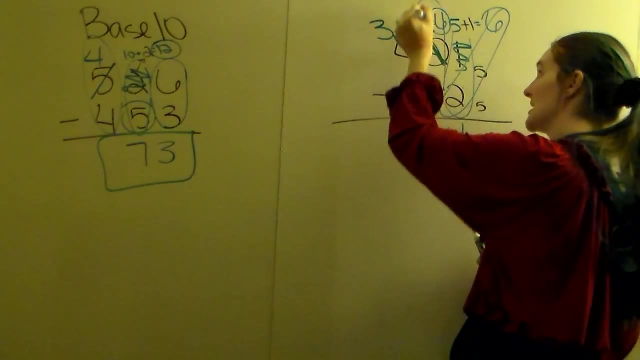 Added to the 1, I'm going to add the base, Always the base. 5 plus 1 is 6.. So instead of 1, I'm doing 6. now, 6 minus 3 keeps us at 3.. 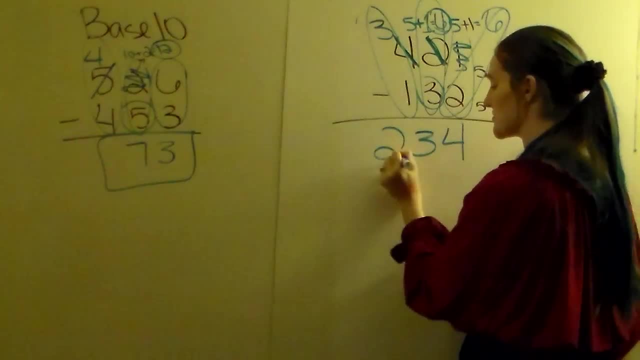 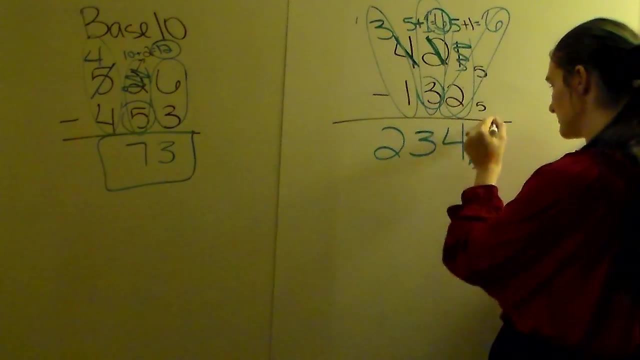 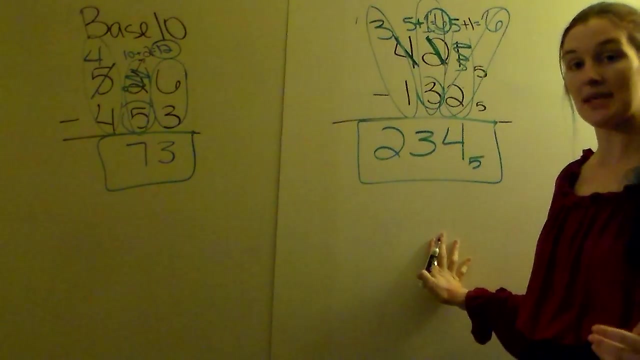 Last column I can do: 3 minus 1 gives me a 2. And the only thing missing is the base. So you don't need to worry about is this number allowed in base 5.. Because subtracting you're always making them smaller.